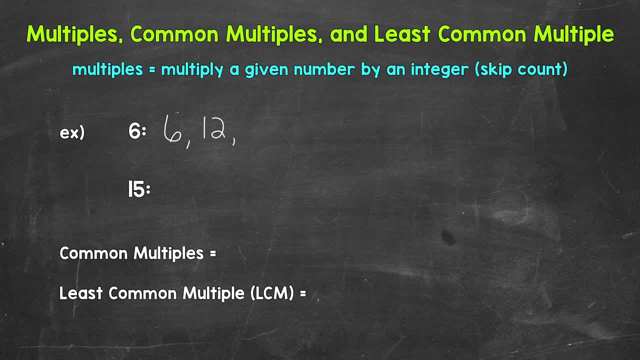 6 times 2 is 12.. 6 times 3 is 18.. 6 times 4 is 24.. And 6 times 5 is 30. So those are the first 5 multiples of 6. And you can see that we just skip counted by 6.. 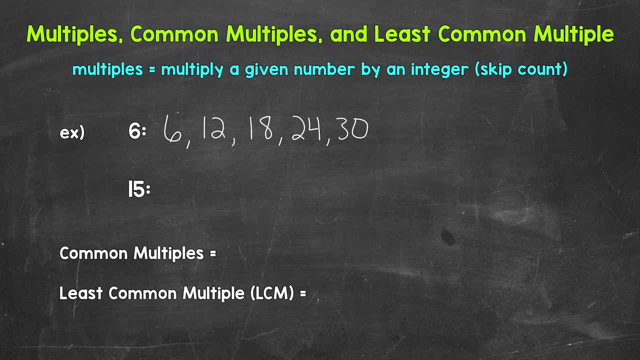 6,, 12,, 18,, 24,, 30, so on and so forth. Now I stopped at 30 because multiples go on forever, They are endless, They are infinite. My suggestion is to list 4 or 5 multiples when looking for common multiples or the least common multiple. 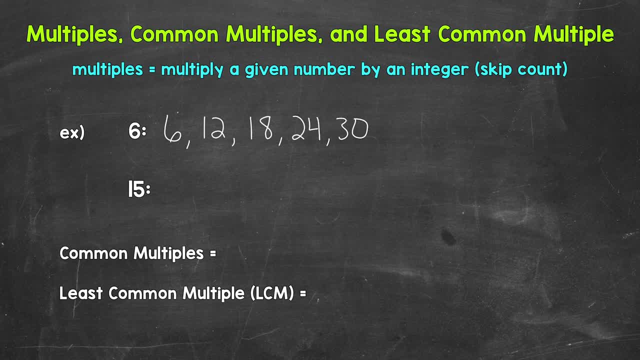 So list 4. Look for any in common, And if you don't have any in common, you can always extend the multiples lists. Now let's list the first 5 multiples of 15.. So 15 times 1 is 15.. 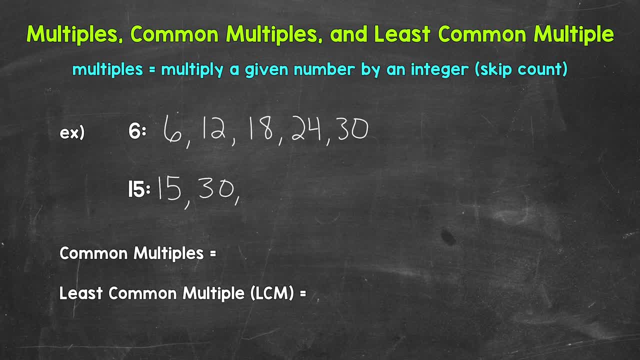 15 times 2 is 30.. 15 times 3 is 45.. 15 times 4 is 60.. And then 15 times 5 is 40. And then 15 times 4 is 60. And then 15 times 5 is 40.. 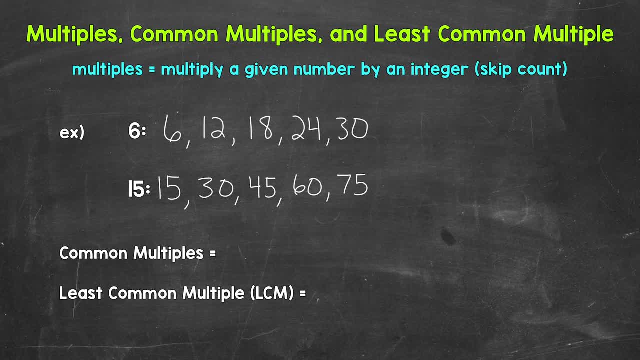 And then 15 times 5 is 75. Now let's look for any common multiples, So any multiples they share, Any multiples they have in common. Well, 30 is a common multiple. The next common multiple is 60. So let's extend the list of multiples for 6 there to show another common multiple. 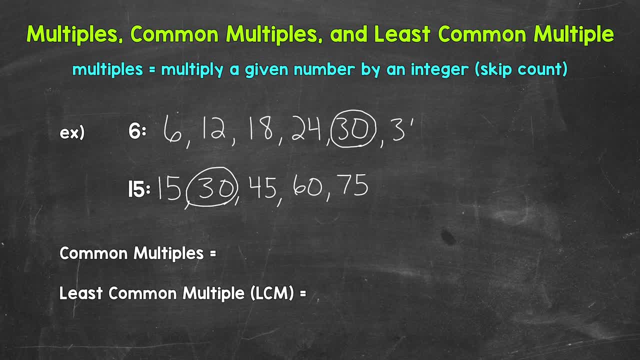 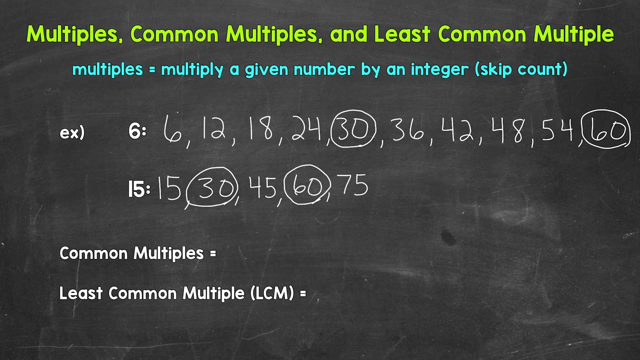 So after 30, we have 36,, then 42,, then 48,, then 54,, then 60. So another common multiple is 60. But again, remember, multiples lists go on forever. So we have an infinite amount of common multiples. 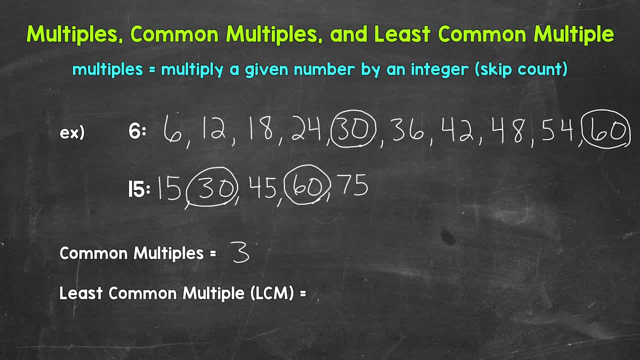 So down below for common multiples I'll put 30., 60. And then make note that we have an infinite amount of common multiples. Now we have the least common multiple, which is just the smallest number in value that they have in common.